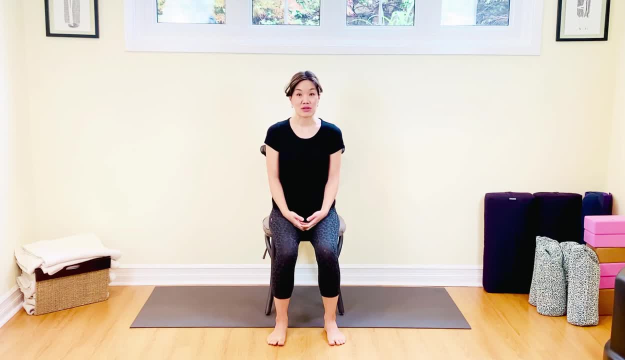 So if you are recovering from any injuries or maybe surgery, you're going to go slow. Okay, you're not going to necessarily do this pace that I'm doing it at. So we're always going to be practicing what is called in yoga ahimsa, which is nonviolence, and that's nonviolence to you. 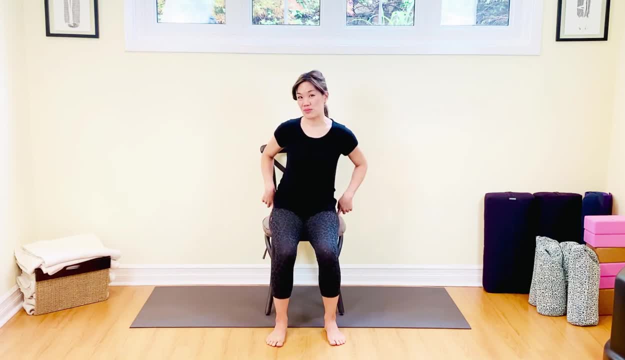 Okay, so in a comfortable seated position with both sits on your chair. we're going to make sure that the chair is nicely planted onto the ground And you'll notice here today that I have it underneath on top of rather a yoga mat, And my feet are going to be planted firmly on the ground. So I'm not very tall, which means I need to come onto the edge of my seat to be most comfortable and to make sure I'm going to be nice and secure. Okay, with my seat sits, bones firmly planted. my feet are planted on the floor. I'm going to spread my toes nice and wide. I'm going to make sure that my shoulders are. 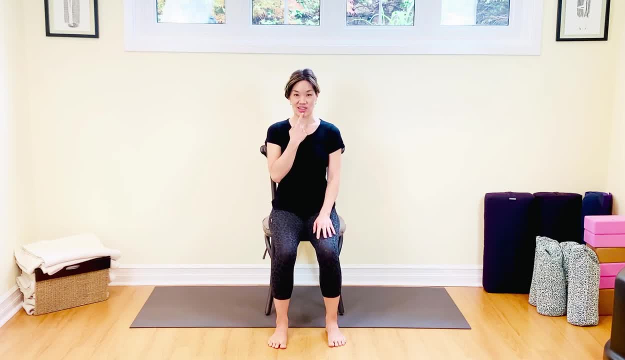 stacked And right on top of my waist and my chin is gently tucked in. That ensures that my spine is nice and tall. I'm just going to take a moment here to start the practice. I'm going to close my eyes. I want you to do this with me and breathe in deeply from your belly up into the ribcage, right into those collarbones, and then I want you to exhale all the way out. 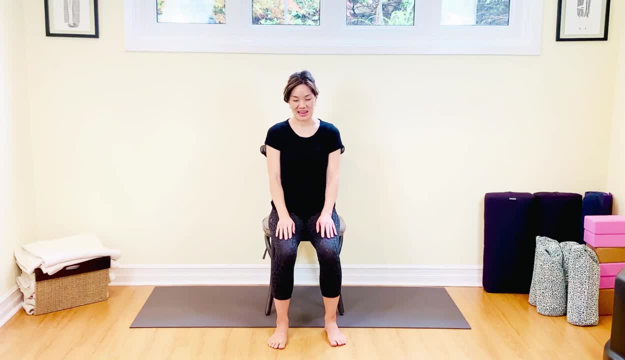 And do that one more time. Oh, two more times, rather Breathing in all the way up, Exhale, relax, all the way out. One more time, Breathing in through the belly, right up into the ribcage and right to your throat, And then exhale, release and relax. 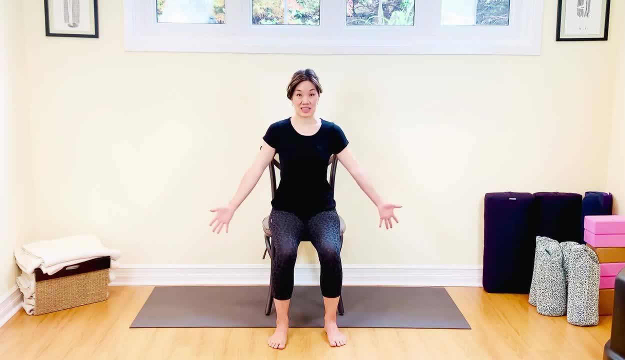 Open up your eyes. Let's take our arms all the way up to the sides, Breathing in nice, big breath. Let's take our hands to the heart, realigning the spine, making sure it's nice and tall. We're breathing in all the way up with those arms and exhale. take your hands to the heart. 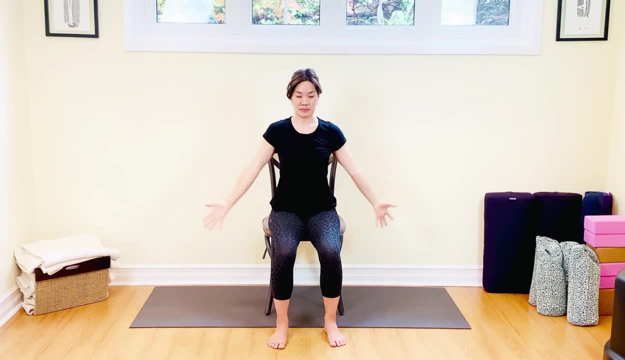 Breathing in again and then touch those fingers and exhale: take your hands to the heart Now, taking the hands up the midline. we're going to breathe in deeply, like this. Breathe in through the spine, Through the spine, through the body: reach, reach, reach. 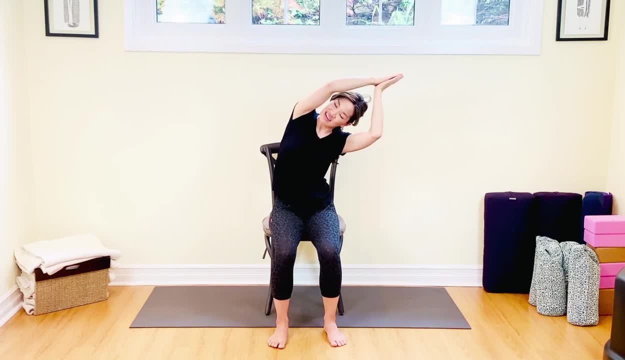 And then exhale. gently. sway to the side. Very good, Keep those shoulders nice and soft, Breathing in back to centre and exhale. We're going to sway to the other side. very good, Inhale, come on back to centre. 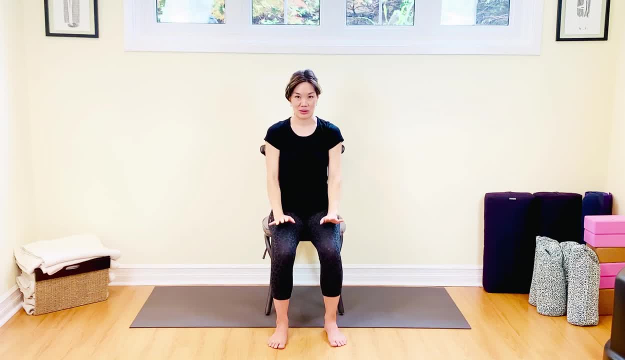 And then let's take our hands down on top of the thighs, nice and slow. So let's pretend we're going to paintbrush a wall in front of us, Breathing in to empty, opening up, maybe looking up if the body feels okay to do that, and then exhale. 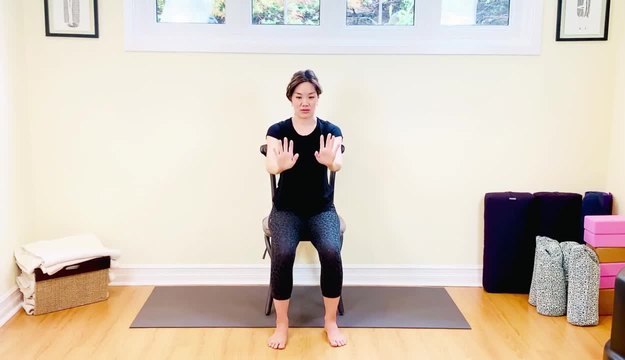 softening paint brushing this wall right in front. soften those shoulders, relax the fingers. breathing in- we're working on expanding our lungs, opening up our chest and then exhaling. softening the arms, relaxing the fingertips. one more time, inhaling, expand, draw the belly, maybe look up and then exhale. soften, relax and see if you can breathe out through the whole breath coming all the way down. awesome, now we're going to take our hands on top of the thighs. let's open up the chest for a seated cow pose. so I'm going to roll my shoulders back, open up my heart and then exhale. I'm going to round my back, bring my fingertips. 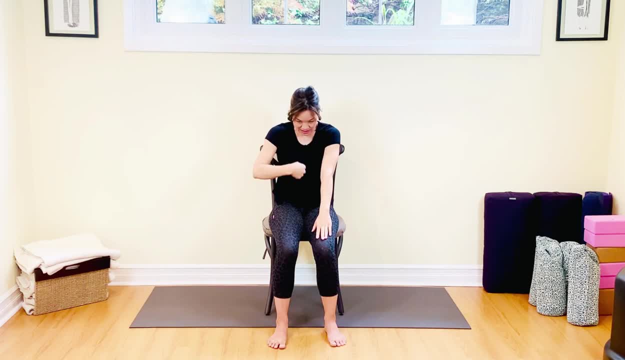 closer to my knees, draw my belly in to the back of the room. draw my chin into the chest, round my back: good inhaling. open up the heart for a seated cow. pose exhale. rounding the back for a seated cat. let's do that a few more. 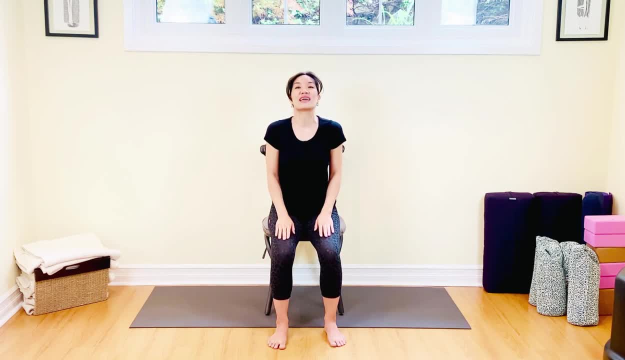 times. think about breathing in from your tail up to your throat and then exhaling breath into the back of the room and then exhale, and then exhale back in, Breathing out from the throat and send it down to the tailbone. Okay, one more time. 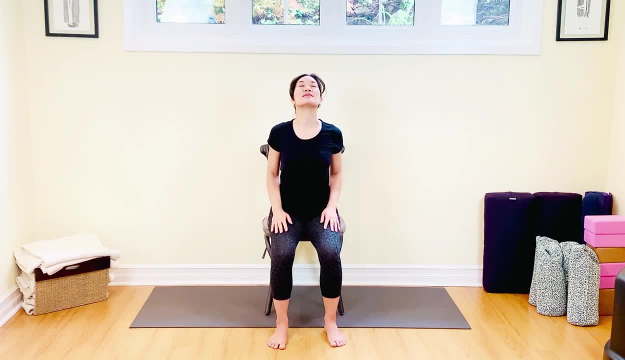 Breathing in nice and slow, articulating that spine, And then exhale rounding the back, softening, please. Very good, Now come on back to that nice flat back. We're going to take our arms down to the sides of us. 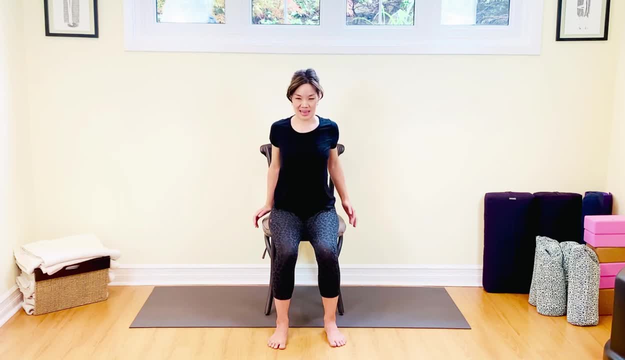 Let's roll the shoulders up and back. I'm going to do this three times, Three times a charm here, Breathing in and out. That feels good. Breathing in and out. Okay now taking your fingertips on top of the shoulders. 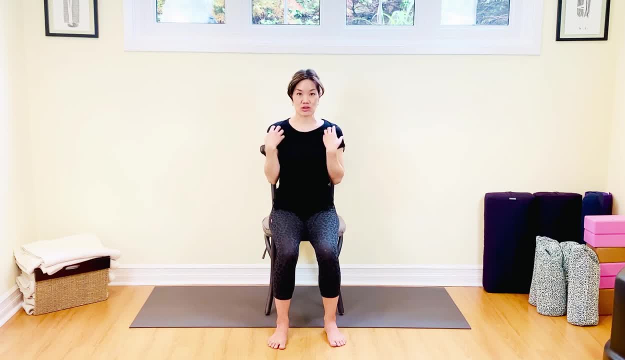 taking the elbows up and around. Now you don't need to be as exaggerated as my arms are going, so maybe they're a little bit smaller like this. So it's your practice, your yoga. You need to do what's best for you. 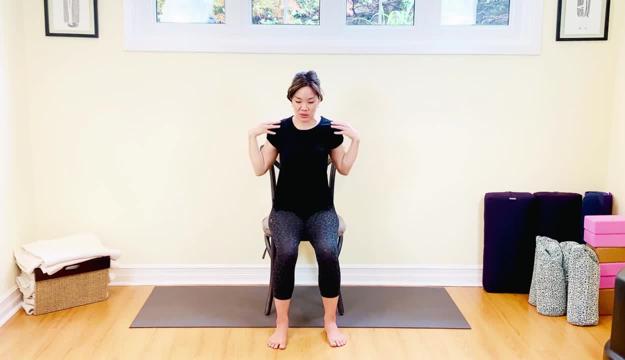 So I'm just always connecting breath with movement. So we're just doing a couple Couple more of these: inhaling, exhaling, breathing in, and exhale, breathing out. Well done, We're going to go the opposite direction. 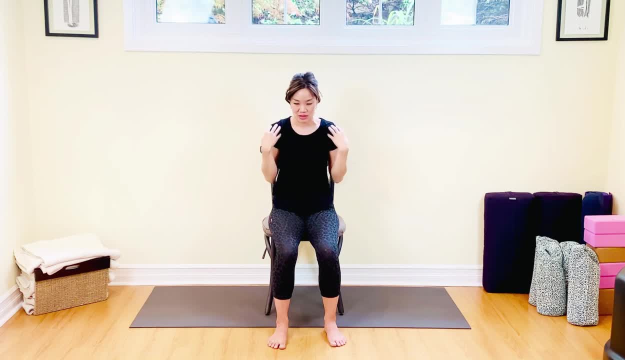 Sometimes this can be challenging, depending on what's happening in the shoulders. Now my fingertips are just lightly touching my shoulders, going up, and I'm going to exaggerate the curl going around Going up, and I'm going to exaggerate a little bit going forward. 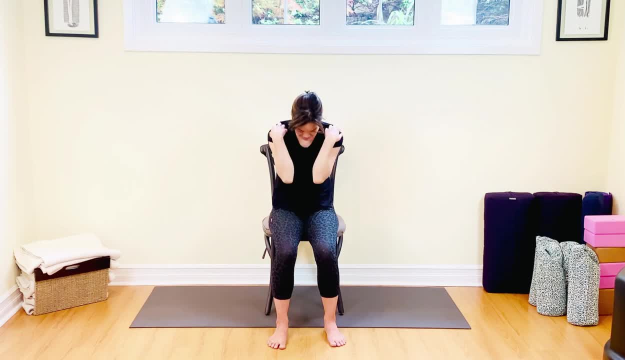 Couple more times: Breathing in, Breathing in and out, Inhale and exhale. Well done, Release the arms here and let's go ahead and take that left arm all the way up. So whenever we take the arm up, I want you to be conscious of keeping that shoulder nice and relaxed. 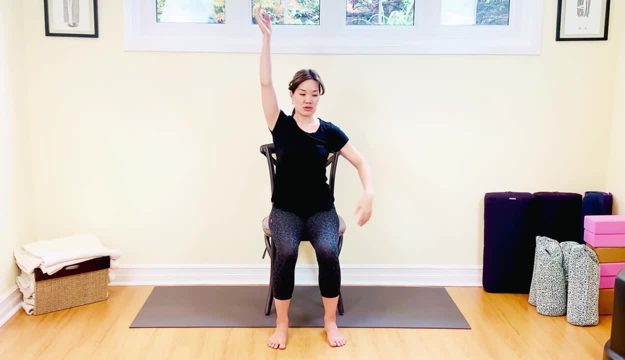 Okay, so we're going to take that arm out. Breathe in, And you'll notice here that I can have my hand on my thigh, or maybe it's securely on top of the chair, or maybe it's down to the side. 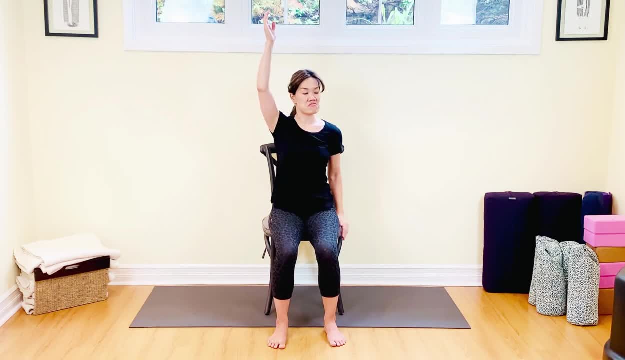 So today I'm going to take my hand. what feels good? I kind of like it on the side of the chair today, okay. So it can be here here or on the side. okay, I'm going to keep mine on the chair, Arms up, lengthen through the spine. 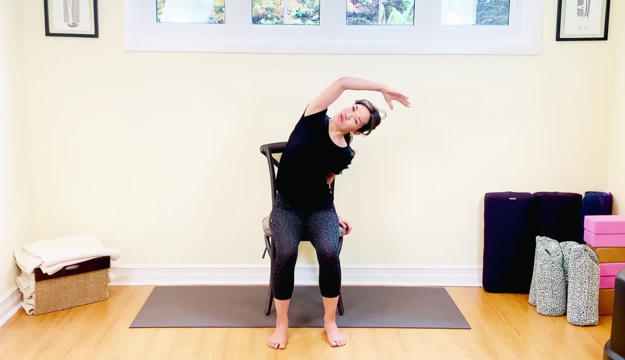 breathe in and exhale. soften breathe out. So when we're swayed to the side- top shoulder and bottom shoulder, even though it's gripped onto, that chair is relaxed, okay, Breathing in. come on back up, exhale. lower down. very good, Inhale, breathing in and exhale. sway to the. 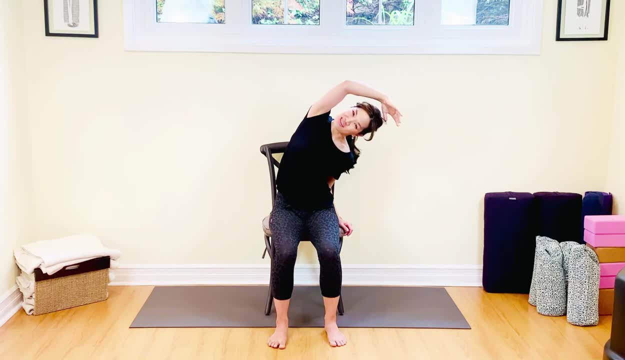 side, soften both shoulders, put a nice stretch to the side of the body- Great. So I did this in my last sequence. I'm going to nudge that elbow up, opening up my chest. I'm going to look up only. 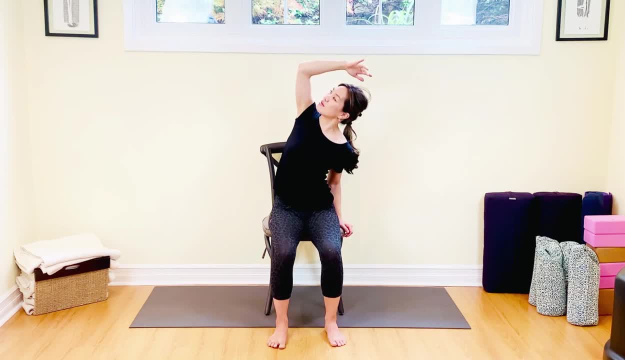 if the neck feels okay to do this. So breathe in, look up and then exhale, Exhale, look down. Very good, Now from here, we're going to inhale, breathe in, lift up, look up. 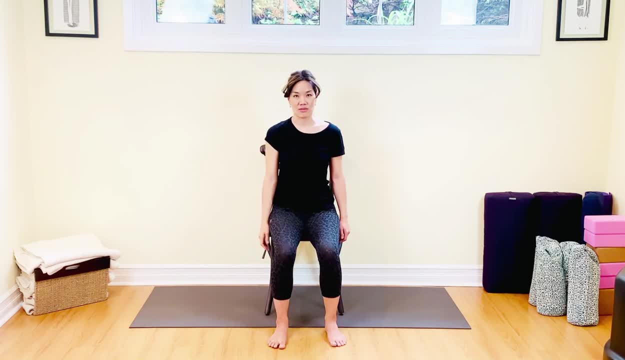 and release, So that arm felt fatigued. So what I'm going to do now is I'm going to shake it out. shake that arm out, okay, Other side now. So I'm going to plant this hand down to the side. I'm. 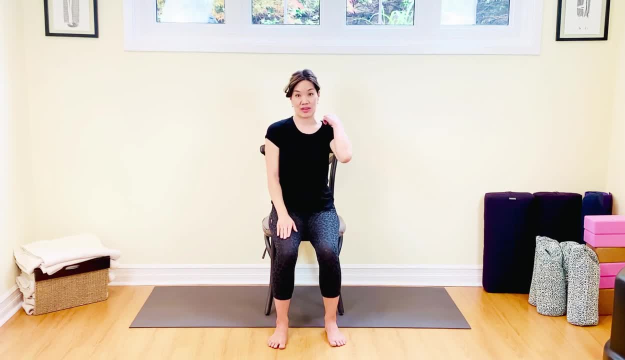 going to equal out the body, So I'm not going to choose to take my hand on the leg or the side, I'm going to put it right onto the chair. so I'm both nice and even I'm going to take the right arm all the way up, relaxing both. 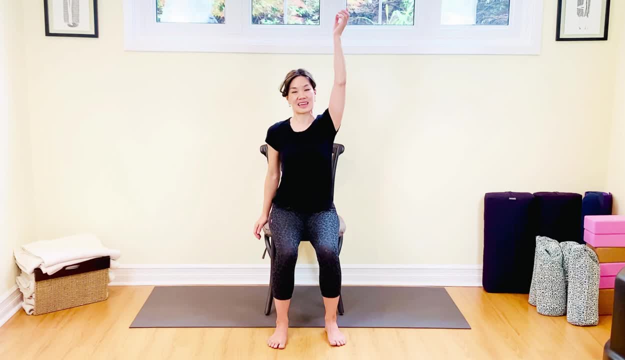 shoulders, drawing through the spine, Inhale lengthening and then exhale swaying to the side. Very good, Keep on breathing. Inhale back to center, Exhale sway. Ah, Always connecting bright lip movement. Inhale back to center and exhale sway. 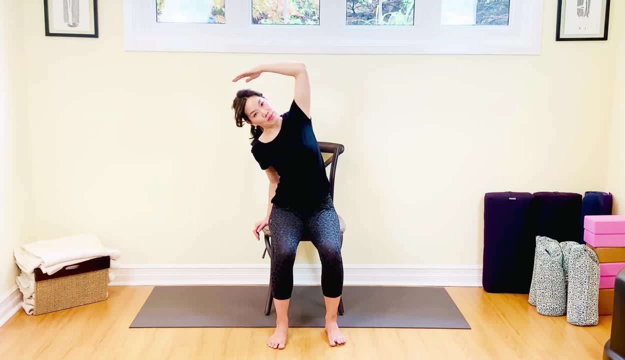 Very good, Now I'm going to nudge that elbow back, keeping that shoulder nice and soft. I'm going to look up, breathing in and exhale softly, looking down to my bottom hand. Very good, Now we're going to inhale, lift up back to center and exhale release. Very good. 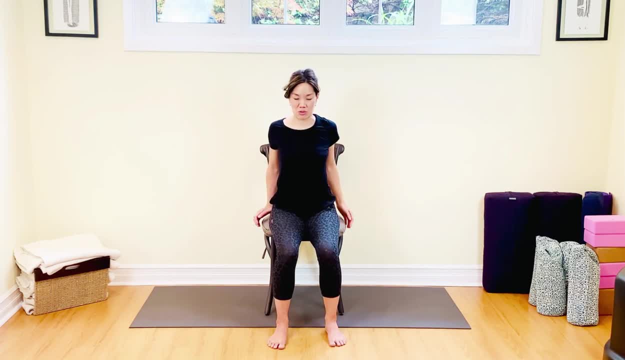 Take those shoulders, Roll them out Very good. Take those shoulders, Roll them out Very good. Take those shoulders, Roll them out times One, breathe two and three. Perfect, Now I want you to take the fingertips, breathe in. 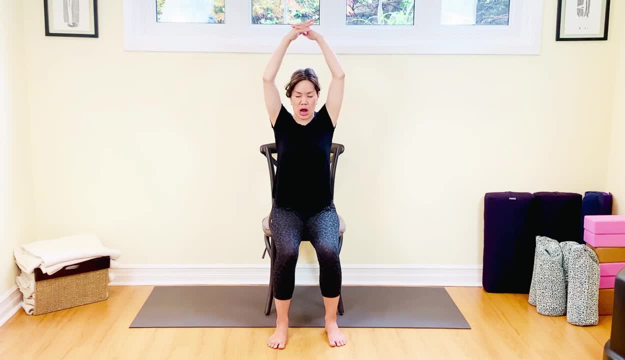 interlace them together and push up Really lengthen out. Inhale here and then exhale. come into that cat pose. We're going to round our backs, draw the belly in, bring your chest in, push those elbows out, contract them and push those knuckles forward. Good, Now we're going to. 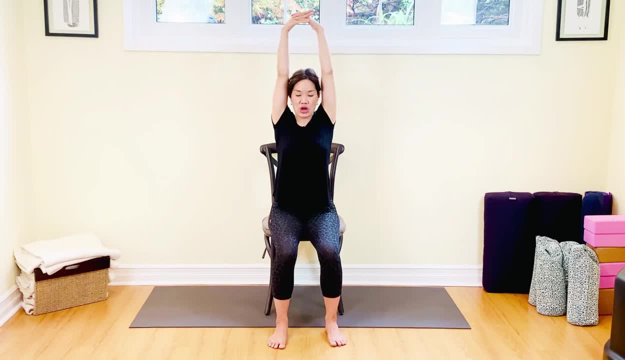 breathe in, lift up, sit up nice and tall. take your hands behind the head, take them open up the chest, expand the elbows to the sides, engage your belly to support the lower back and look up gently. Breathe out. 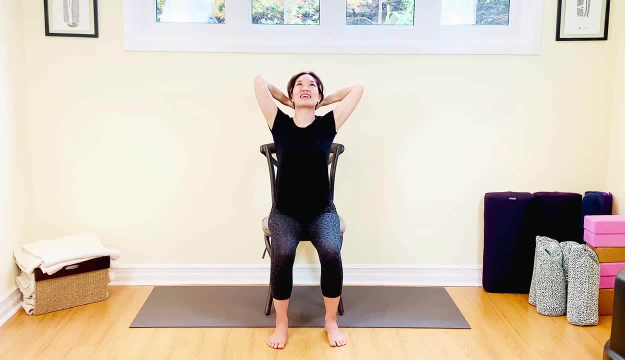 So you're just in a nice holiday position. We're going to do that again. We're going to come back to center, breathing in, undo those fingertips, breathe out, release. Okay, we're going to do that two more times. So, breathing in, interlace, the fingers breathe out, inhale, lift and then exhale. 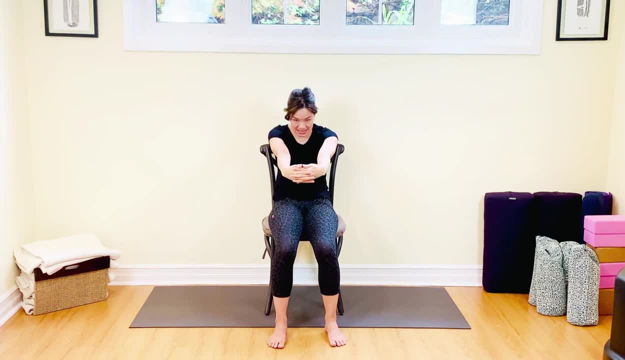 round the back With a nice tight belly. come on up, Inhale to lengthen up and take your hands behind the head, draw the belly in, lift your heart up to the sky. Awesome Inhale back to center. 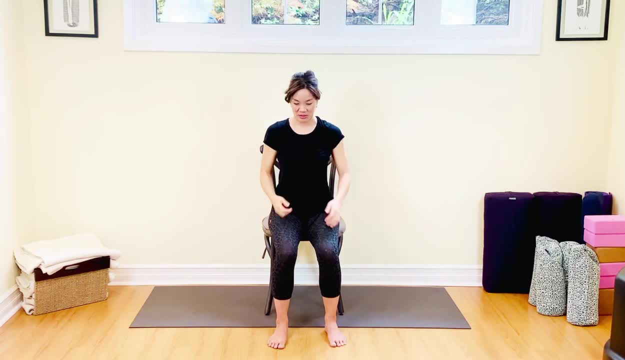 and then exhale release. Last one: We're going to breathe in arms up, interlace them, breathe out, relax the shoulders and elbows, Inhale, extend, breathe in and then exhale round the back. 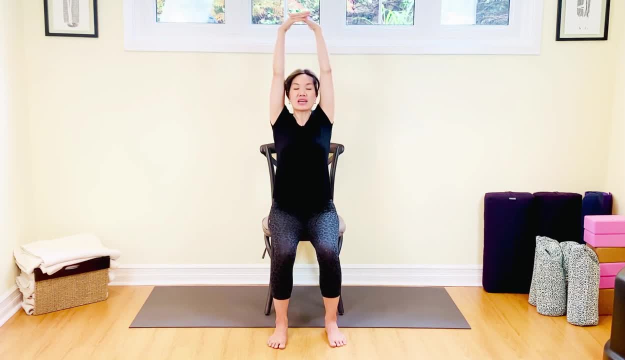 Great Breathing in. lift up chest up, draw the belly in and then exhale round the back, Inhale back to center and then release, Breathe out. Well done, Okay. Now how about we shake out? 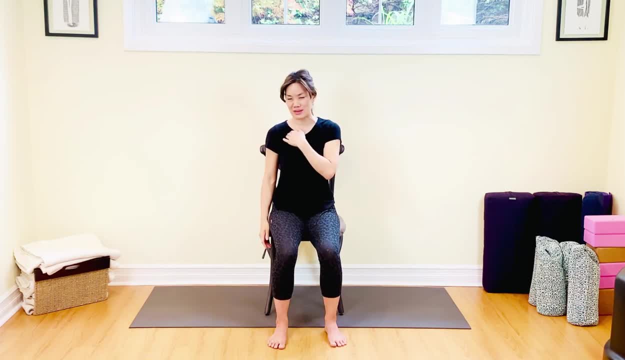 those arms. I shook it out on that one side because that's my grumpy side, But why not shake out both of them? And as I've done in other classes and you know that I am an acupuncturist- 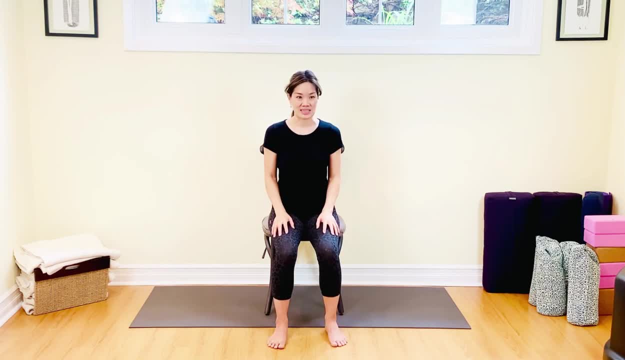 I'm all about that chi and the meridians, So I like to tap on my body, So I'm going to ask you to go ahead and tap onto your right shoulder, So it's going to sound like I'm tapping pretty hard, because I am. I need a good shoulder massage. 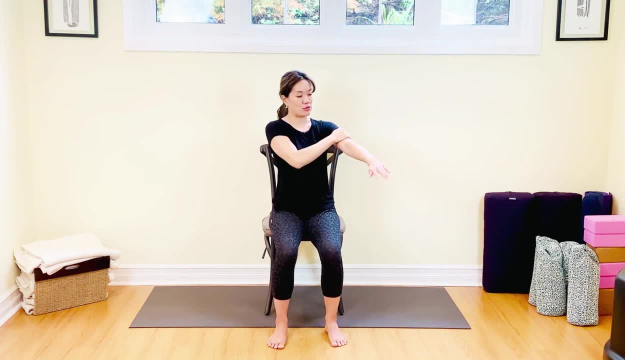 Okay, So I'm going to tap onto my shoulder. I'm going to tap all the way down, So you're going to see that I'm tapping pretty firmly. Then I'm going to tap on the inside of my arm. Really, tap it nice and hard. Now your choice of how much you want to tap or how heavy you're going to go. 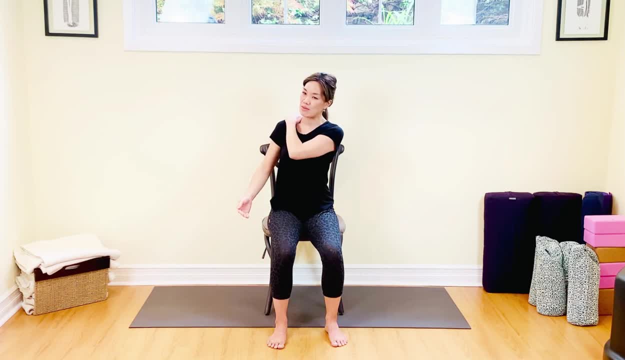 So it's not a no pain, no gain situation. You're just going to tap to stimulate the yang and the yin parts of your body. So I'm going to go down and ask you to tap on the inside, coming all the way back up. Very good, Now that I've done. 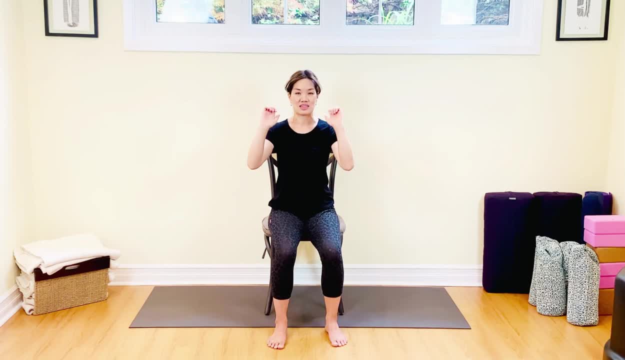 that part. I'm just going to ask you to tap gently. I'm going to close my hands in a gentle fist and just tap right here. So it's right under the clavicle, right under your collarbones. Give yourself a nice tap, Take a breath in. 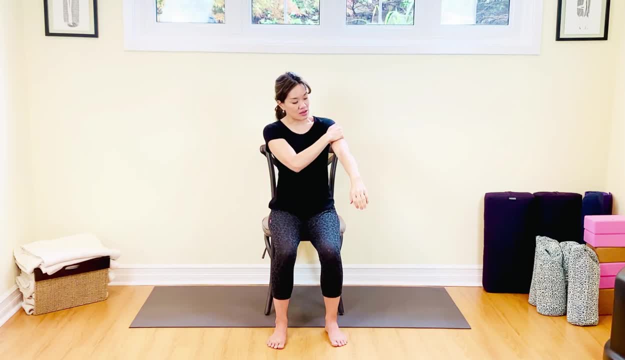 Perfect Release. I want you to gently or firmly, your choice- press on the outside of the body Down and up. Come across all the way with gentle or firm pressure Down and up and across. I'm going to do that again. Three times a charm here. So this is number two: Pressure. Just enough, Okay. 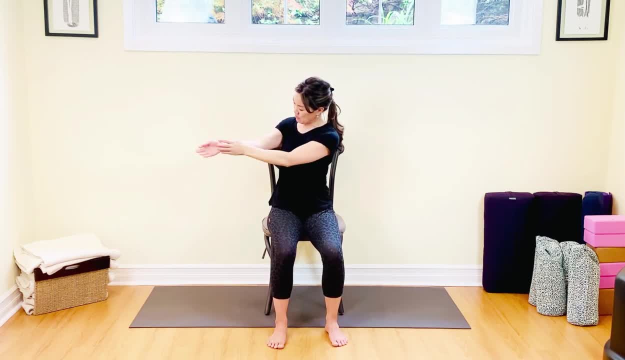 And across. This is three: Perfect, Awesome. I'm going to shake out my wrists. I really want this to be a full body stretch. I'm going to roll out the wrists Outward. Now I'm going maybe a little too fast So you can go slower. You need to go slower, Go slower. I'm going to go inward. 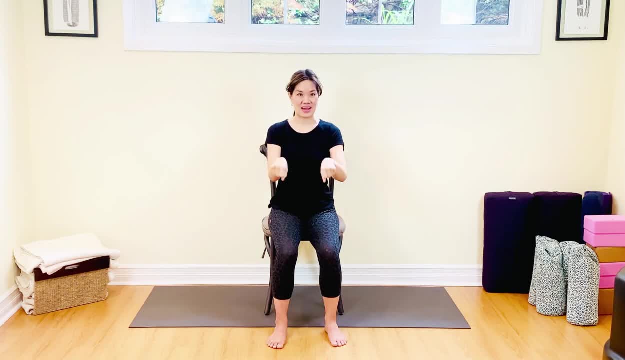 It's interesting how the body is. If you're going fast, then maybe the mind is racing a little. Okay, Now I would like you to do your piano playing. So go ahead, Don't forget those thumbs, Those thumbs. Go ahead and play the piano And then let's do the grand piano from right, all the way. 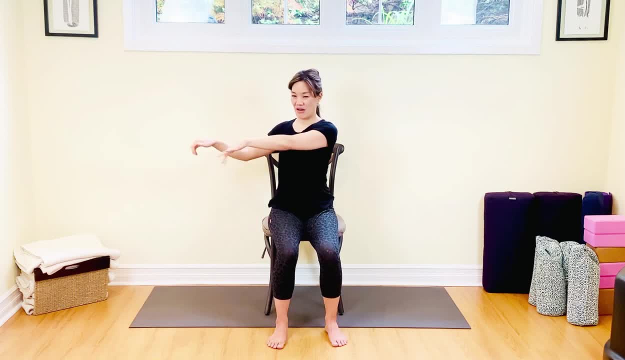 to the left. Don't forget to sit nice and tall All the way right to left. And this is a perfect little segue because we're going from right to left Now. it's a perfect segue to do our twist, So it's release Perfect. 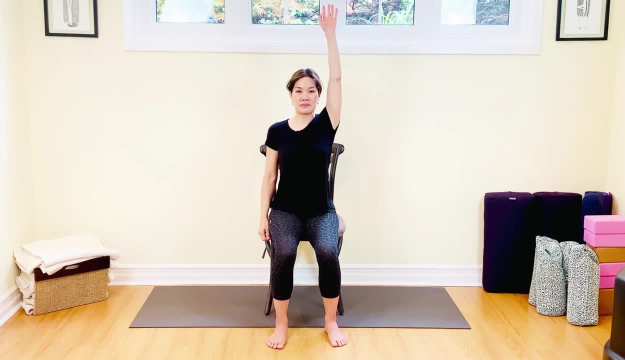 Now let's take the right arm all the way up, Breathe in here And then exhale release. We're just getting used to our arms again Breathing in, Lift And then exhale release. Okay, So now we're going to take the right hand, Place it nice and firmly behind you on the chair, On the seat of. 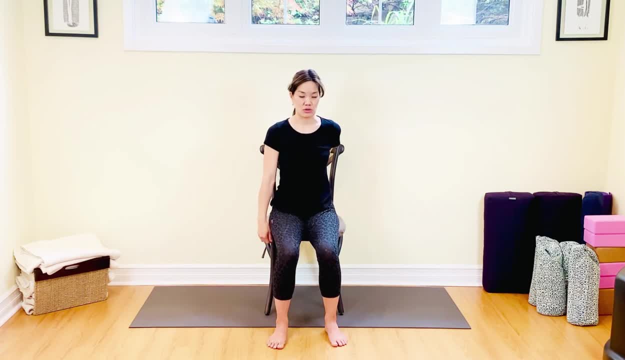 the chair, if you can. Okay, So it's nice and close to your tailbone. I'm going to take the left arm all the way up. Sit nice and tall, Breathe in here And then exhale. Take it to the. 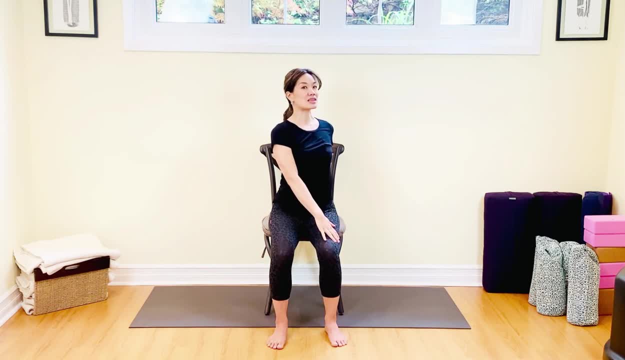 outside of that right leg. I want you to inhale, Lift and lengthen through the spine, Keeping your chin right on top of the sternum. Breathe out Twist, Relax your sits, bones, Relax your shoulders. Inhale, Lift and lengthen. Exhale Twist Again. Inhale, Lift, Lengthen And then. 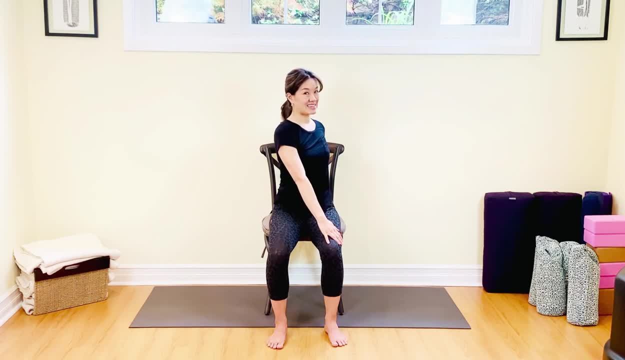 turn them. Breathe here In, Now exhale. See if you can turn your head to look behind you. Inhale here And then exhale. Stay in the twist. Look over your opposite shoulder. I always like to. 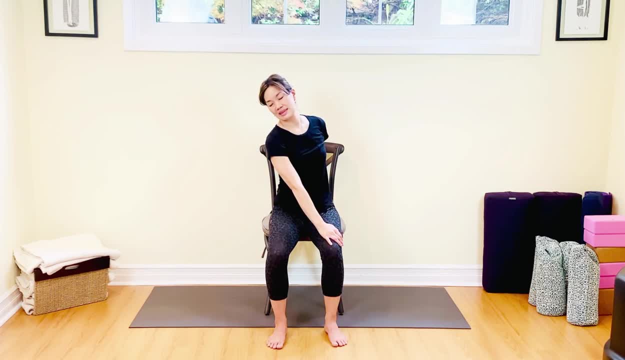 close my eyes in these gentle twists. Breathe in And out Helps me to relax my shoulders even more. One more breath here, Breathing in And out, Now to come out of the pose we're going to inhale And then on the exhalation. 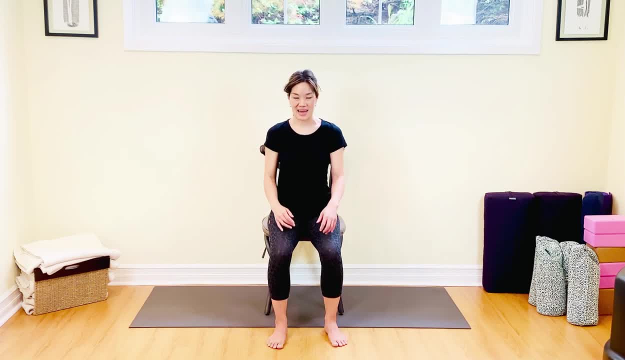 we will unwind, Breathe out, Come back to center- Fantastic. So now we got that hand behind, We're going to take this left hand, Place it down behind us And notice how I'm trying to keep this back shoulder nice and relaxed. Inhale, Lift And then exhale, Taking that hand, the right hand now. 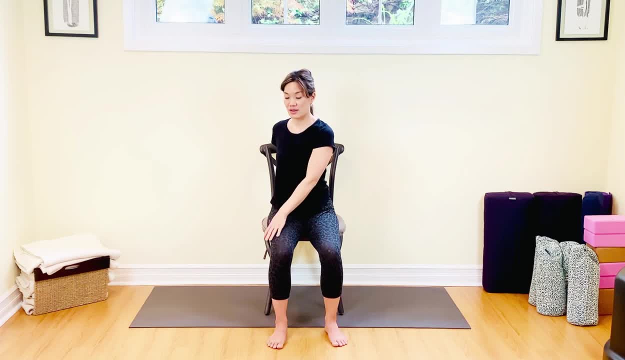 on over the shoulder And then exhale, Taking that hand, the right hand, now on over the shoulder, And then exhale, Taking that hand, the right hand now on over to the left side of that, or the outer edge, Rather of that left leg. Okay, we're going to breathe in, lift, Lengthen And then exhale Gently. 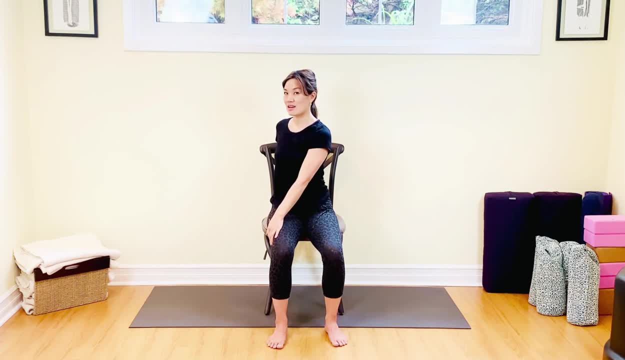 twist, So don't grind your sit bones into your chair. Relax the hips, Breathing in, Exhale Twist, Keeping my chin right over my sternum. So I'm keeping. I'm really kind of working and twisting in my thick bony part of my spine, The thoracic part, Breathing in. 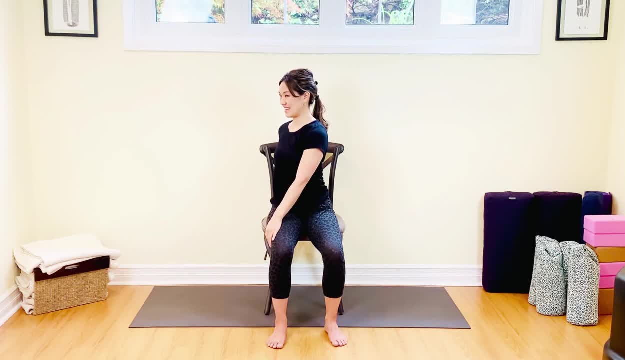 and exhale. twist, good now. inhale here, chin right over the sternum, and then exhale. let's go ahead and see when you look behind us and then inhale. stay in the twist and then exhale. see if you can look over the opposite shoulder. relax. 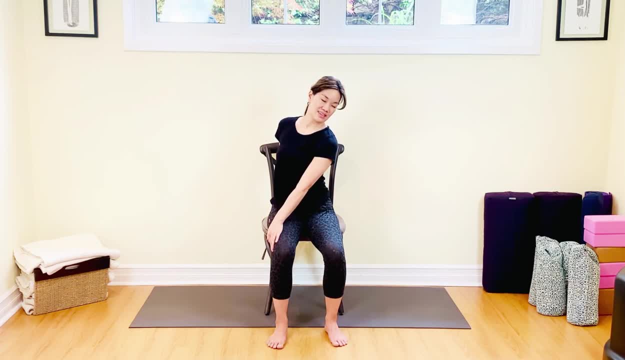 your body and the shoulders. you're still in that twist. close your eyes, if you can, to really enjoy this twist. breathe in and out, inhaling. exhale in and then to unwind, breathe out, unwind. come back to center. well done, take the hands right on top of your head and bring them back to the center, and then bring them back to. 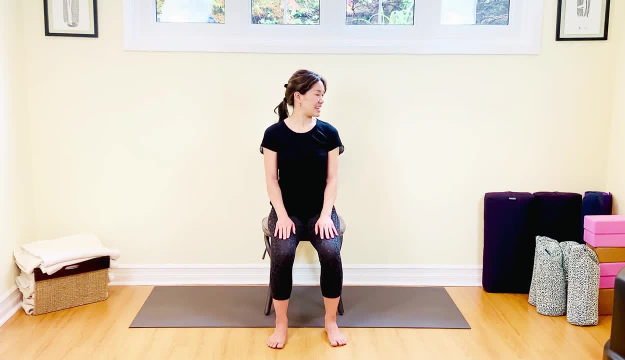 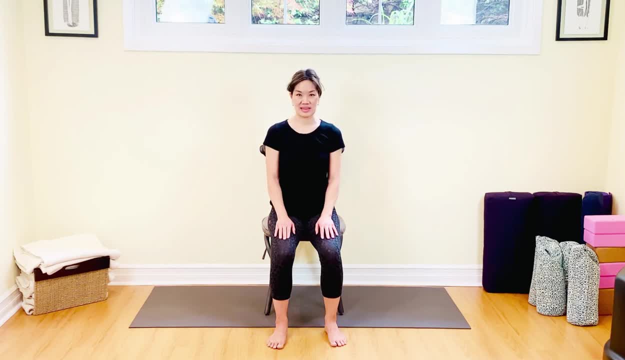 look over to our right again- I'm sitting. look over to our right again- I'm sitting. nice and tall. come back to Center. let's nice and tall. come back to Center. let's nice and tall. come back to Center. let's look over to the left- is everybody. 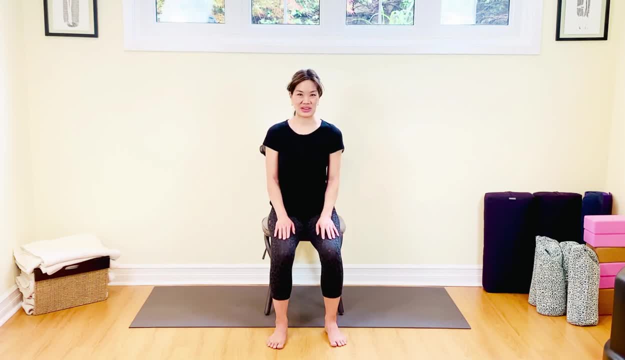 look over to the left. is everybody look over to the left? is everybody breathing? come back to Center now, let's breathing. come back to Center now, let's breathing. come back to Center now. let's go ahead and take that left ear to left. go ahead and take that left ear to left. 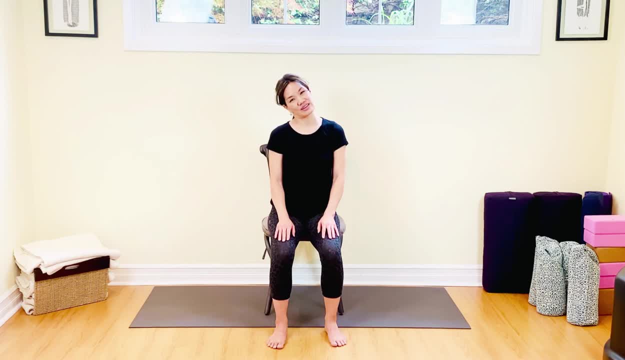 go ahead and take that left ear to left shoulder. oh, my neck is super stiff today, shoulder- oh, my neck is super stiff today. we're gonna try to relax here and then to send more, a little bit more oomph into this little stretch. I'm gonna send energy through these fingertips outward. 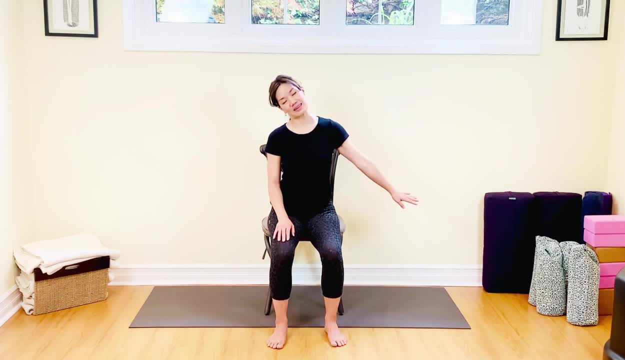 keeping my chest open, my back flat against that imaginary wall behind me, and I'm doing this nice little stretch here, inhaling, and then whoo, exhale, release, release the hand, release the neck. let's go ahead and take it to the other side. is this your comfy side or is this just as good as the other side? 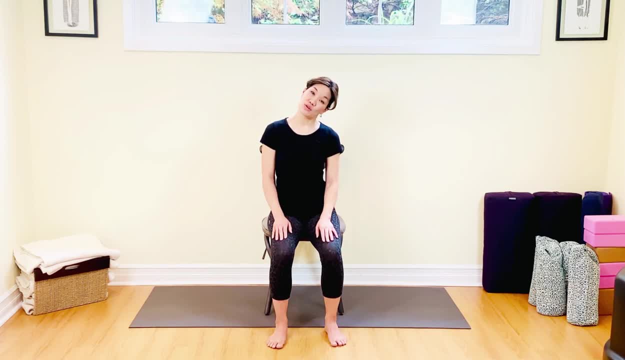 take that here and then, if you want to eat, this is good or not good, let's go ahead and some energy out of those fingers send energy like this, electrical rays going out of those fingertips, breathing here in and out, inhale and then exhale, let's release, come back. okay now, if you always want a little bit more in those, 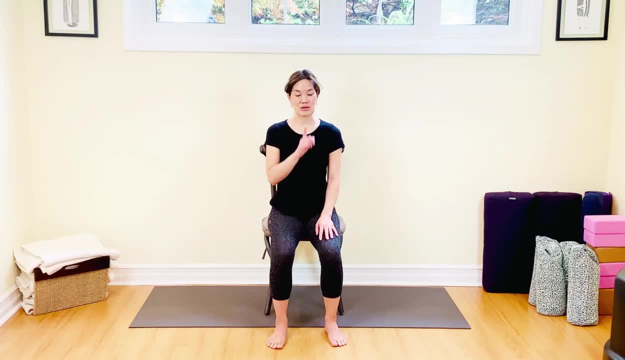 stretches. feel free to do something like this. we're gonna go back on to that side. okay, now that we have the hand is pretty heavy, so I'm just gonna place it on top of the head. notice how that may change a little. so then that's. if you wanted a, 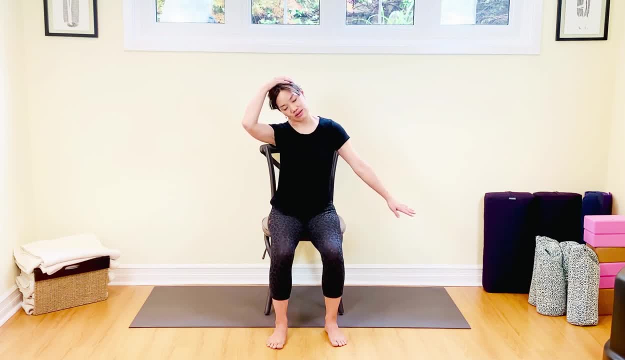 little more and then taking the hand out, sending energy through those fingertips. now, something a little bit different than I've done in my past sequence: I'd like you to lower the hand down, releasing the hand from the head. I want you to turn your head to look down to your left hip. taking your hand now to 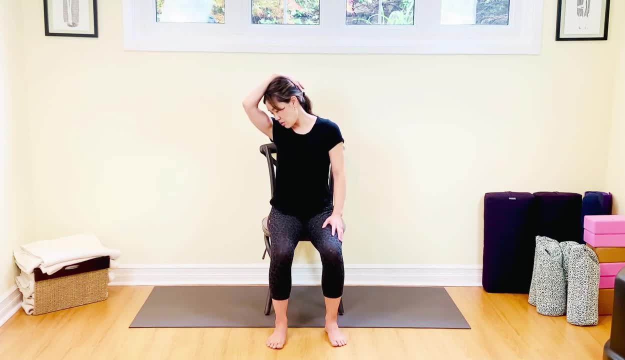 the back of the head. we're not pulling or putting any major pressure, just the weight of the hand in the arm. it's gonna do a nice gentle stretch and the back of the neck and the side breathe here, gazing down to the hip, relaxing. good, now we're going to release the hand down, like you, to breathe in. 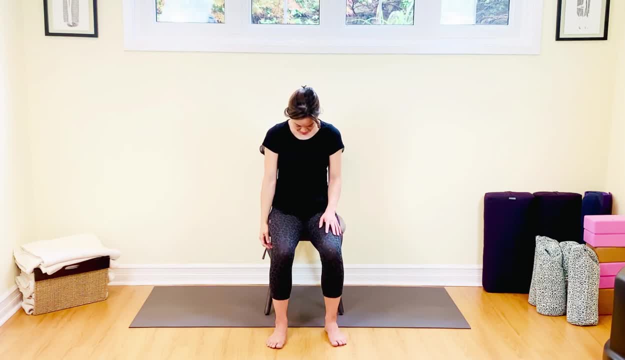 look down to Center, breathe out and then inhale, look up and then exhale, release. ah, okay, let's do the other side lower that head down. whoosh good, good, okay. let's do the other side lower that head down. whoosh good, good, okay, let's do the other side lower that head down. whoosh good, good, okay. now again you don't have to do. 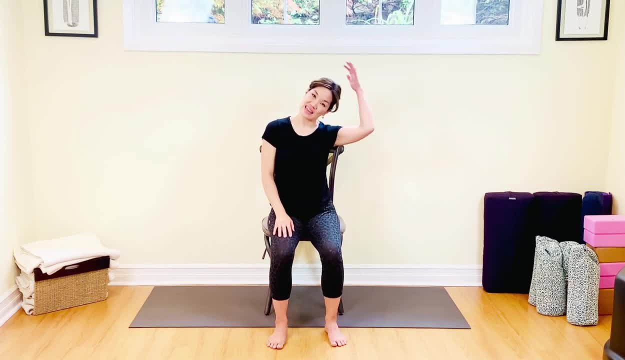 okay, now again, you don't have to do. okay, now again, you don't have to do this. this is it only if you want a little bit. this is it only if you want a little bit. this is it only if you want a little bit more. you take the hand on top of the. 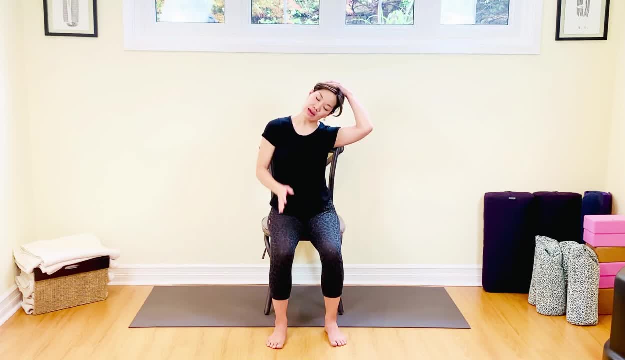 more you take the hand on top, of the more you take the hand on top of the head. because my hands pretty heavy, okay, head, because my hands pretty heavy, okay, head, because my hands pretty heavy, okay, and then we're gonna extend those, and then we're gonna extend those. 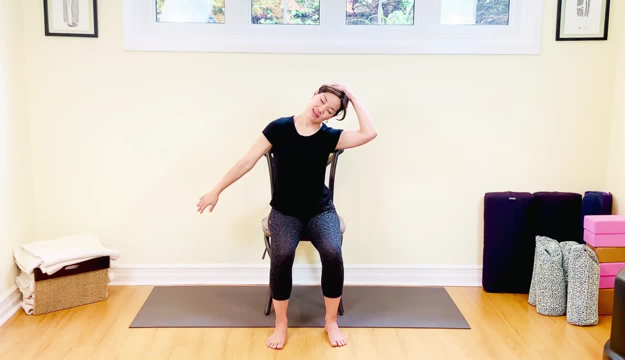 and then we're gonna extend those fingers. send the energy now, please don't fingers. send the energy now, please don't fingers. send the energy now, please don't crank your neck. just the gentle weight crank your neck. just the gentle weight of the hand is more than enough. release the hand down. release the hand above, turn your head down. 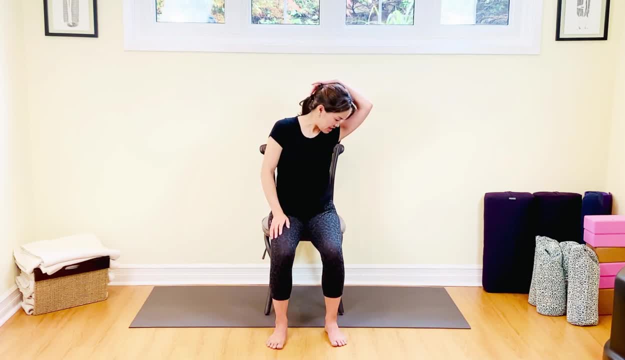 to look to the hip and take and place your hand to the back of your head and then place it on the head and you will feel a gentle stretch. breathe here, in and out, through the nose, gazing at your hip, shoulders relax, inhale, exhaling, releasing the hand, breathing in, looking to center. 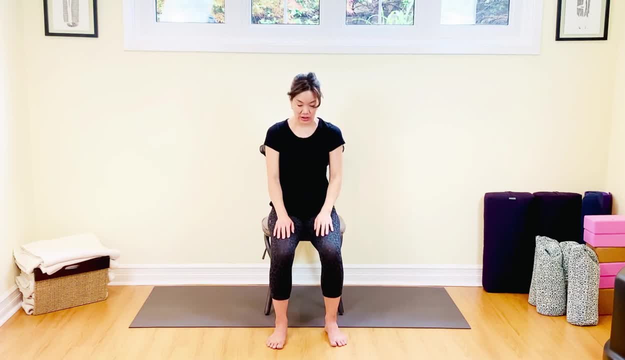 and out. now inhale. look up, always breathing in when you look up and then exhaling how you doing. okay, so now we're going to take our hands to the sides of the chair. let's go ahead and work on our lower body. okay, so feet, making sure that they're planted on top. 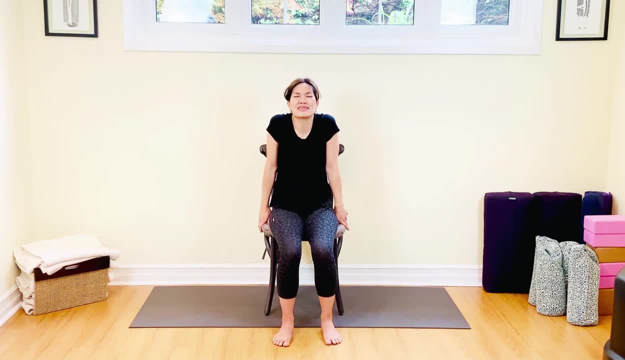 on the ground here. i don't want there to be shoulders into the ears, no, no, no. we want to relax the body, but sit nice and tall, nice chin tuck okay. so the back of the neck is long okay. so we're feeling strong and supported. let's go ahead and take that right leg up, the knee up and release. 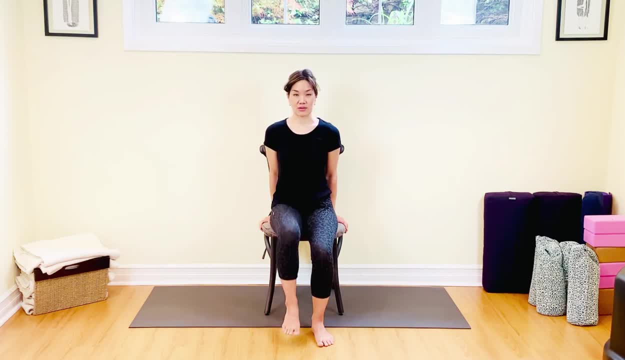 other leg up, inhale and release. now do you want to take your hands to the front on the side and see if that changes anything? you will need to work on your core stability here. inhale and exhale so you see what's best for you in your practice. in all cases, we're drawing the belly in to support our spine in. 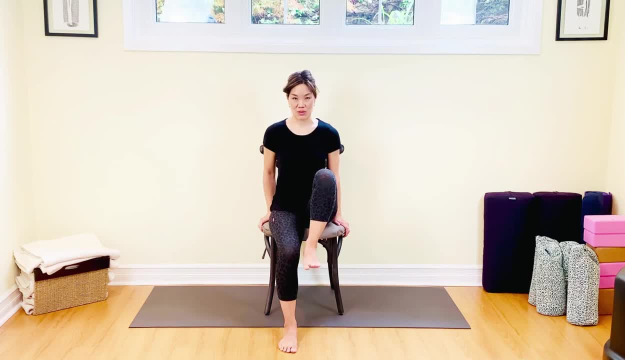 the back. we're working on core strength, but we're also doing nice low compression here in our psoas- groin muscle, our inguinal area. okay, so is everybody breathing? perfect, we're gonna inhale and exhale. now with support. we're having our hands to the sides or on your thighs. breathe in. 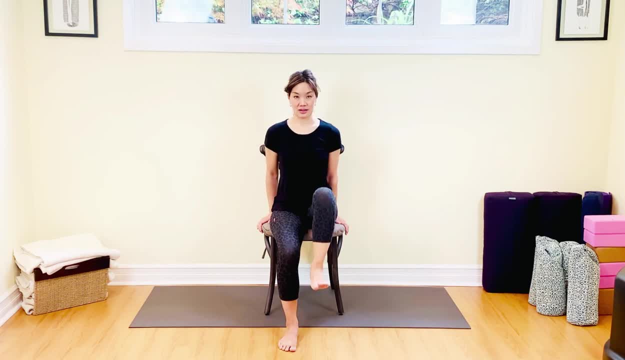 and then let's kick it out. breathe out, inhale and exhale- okay, breathing in and out. inhale and exhale. okay, inhaling, exhaling. you noticing how you need to really engage your belly muscles, strengthening the core and your spine, your back muscles in and out, chest up open, nice and straight in and out. we're doing. 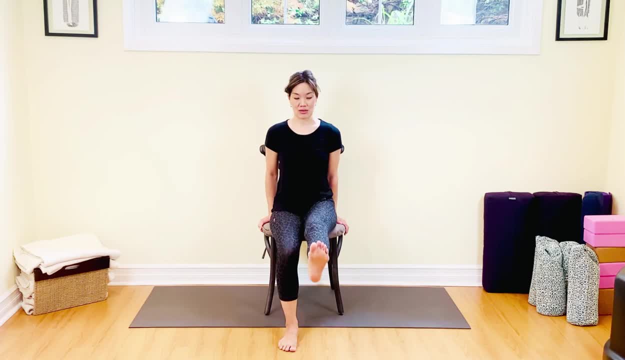 one more set, can we go? breathe in, extend, breathe out, inhale and exhale, inhale, exhale. breathing in and out. well done, now i'd like you to take your arms all the way up, breathing in, touch your fingertips, breathe out. take your hands behind you on that lower lumbar spot. i want you to rub it. 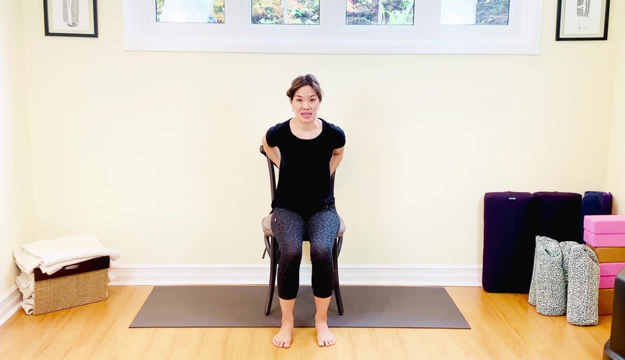 and warm up that lower back nicely where your kidneys are. okay. now i want you to breathe in, open up the chest and then exhale. we're gonna come down dead. as we've done before in my last session, we're going to take the hands down to the sides of the body, Breathe out With a nice tight belly. 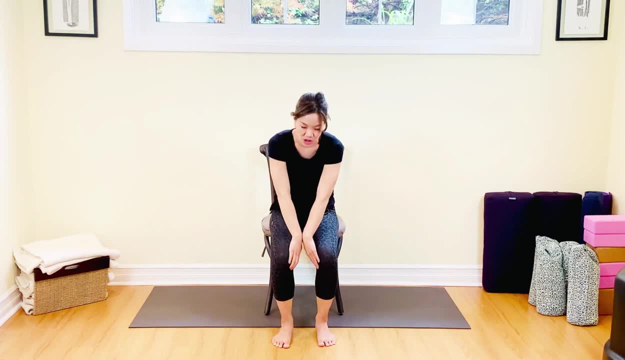 I'd like you to take your hands on the inside of the legs, gentle pressure. So we're doing the whole yang and yin thing that we did on our arms. okay, We're going to do that again: Breathing in, touch. Breathing out Inhale as we rub and warm up our lower backs. Breathing out Inhale. 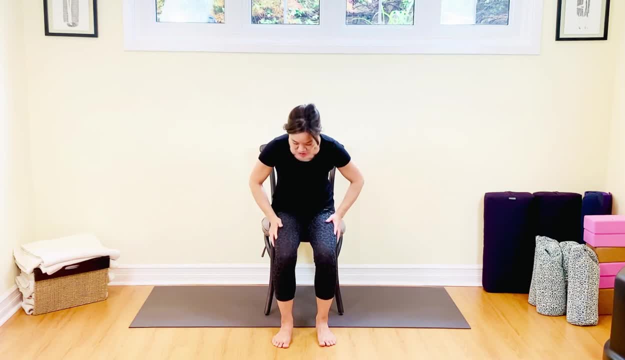 open up the chest And then exhale gentle pressure on the outside of the legs. I want you to press, press, press And then breathe in hands on the inside of the legs, Press all the way up. Okay, We're going to do that one more time: Breathing in, touch, Breathing out. Inhale as. 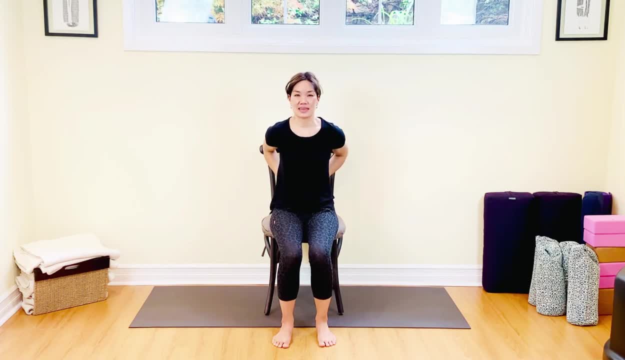 you rub Exhaling, Inhale. open up the chest a little And then exhale. We're going to come all the way down. Breathe And then inhale, Of course. tighten up those belly muscles, Press on up, Come on up, And then let's go. 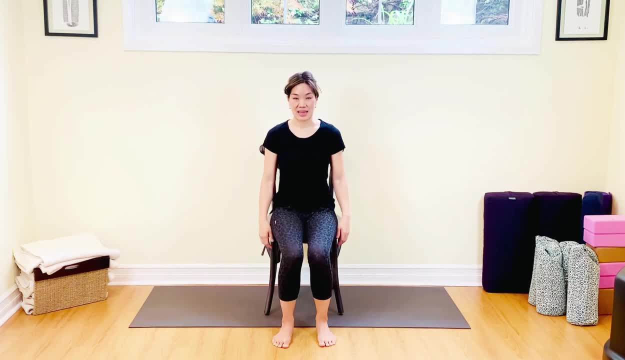 ahead and roll the shoulders back- Well done, Okay. Taking your hands down on top onto the sides of the chair. Let's go ahead and give that leg a little shake And then switch. Let's go ahead and shake that too. Now we did tap on our arms, didn't we? And do that nice little rubbing. We're going. 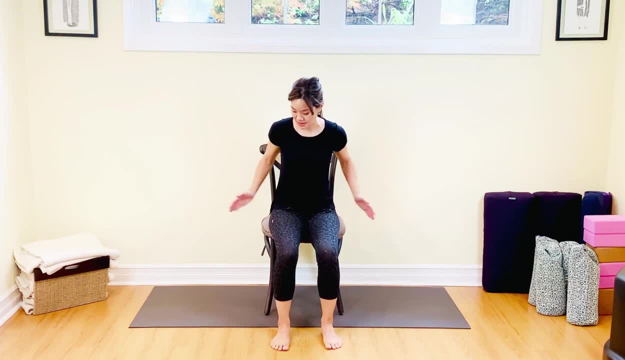 to do that on our legs as well. So go ahead And tap on the sides of your hips. You're like, okay, she's making me tap onto my butt. Well, a little bit of your butt, Okay. So the gluteus maximus medius are your biggest muscles of the body, And for those, 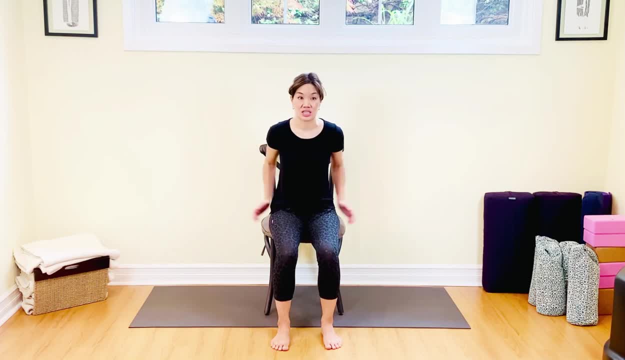 of you who are sitting a lot. well, they take a good. they take a good beating sometimes. So now you're actually going to beat them to some degree. So you're going to have a little, a little or a lot of pressure with a nice tapping, And I want you to go ahead and tap on the sides of your 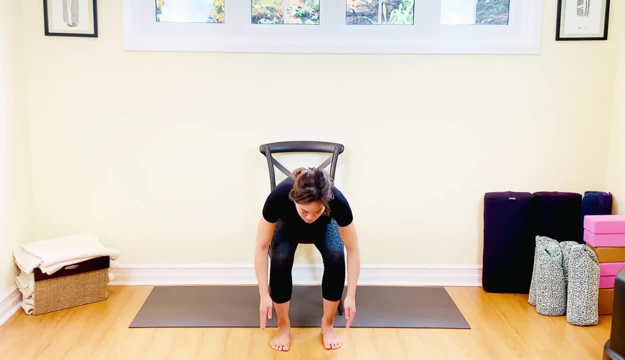 legs. Let's go ahead and stimulate those young meridians, And let's go ahead and tap on the inside of the legs too, Gently. So every time we do that, we're going to breathe out as we go down, And then we're going to. 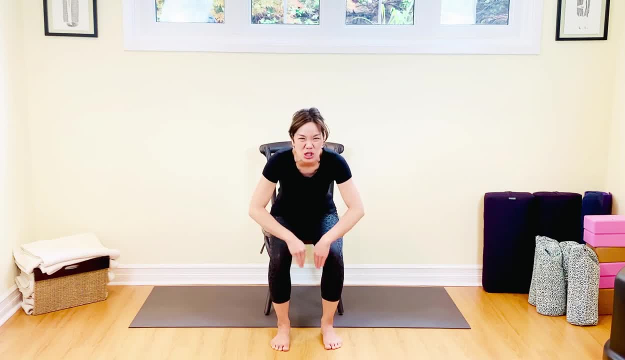 inhale as we come on up And I'm going to tighten my belly muscles to support my spine as I come up. Okay, I'm going to do that one more time, Tapping And all the way down, Breathe out And then inhale with a nice tight. 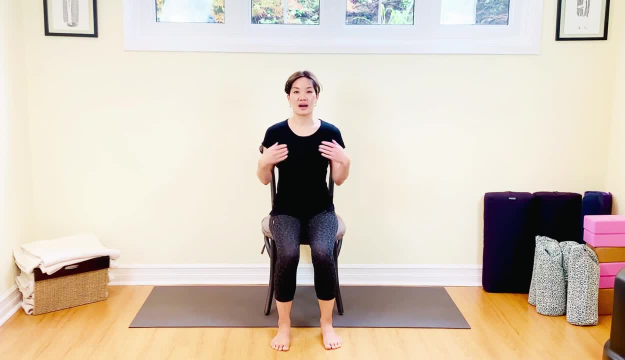 belly, Come on up. Well done Now. hands to the sides, Please. let's go ahead and lift up Back straight, Lift up that right knee, Breathe in, And let's go ahead and cross that leg here. Okay, Now taking your fingers. 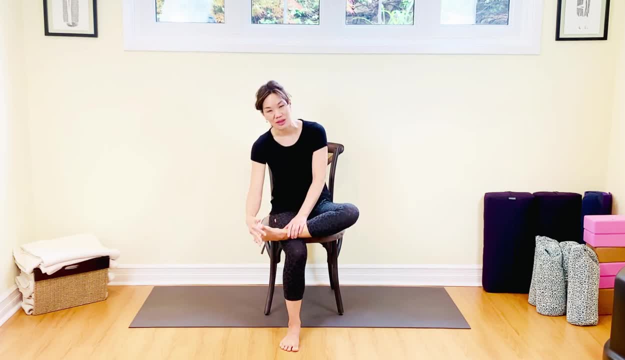 and see if you can interlace your fingers with your toes. Your chiropodist or podiatrist, I'm going to love you for this. So think of yourself as interlacing those toes. And not everybody can get those fingers in between those toes. nice and easy. 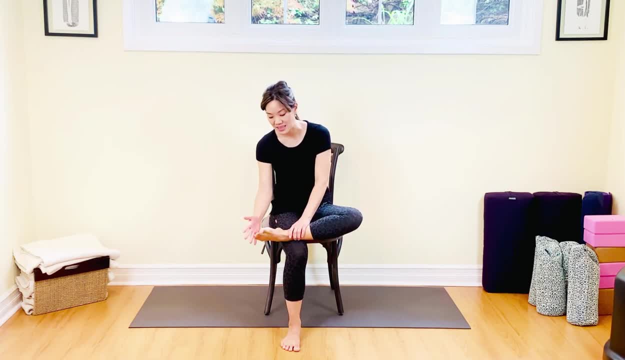 So this is something that you may want to start working on: Go ahead and see how much you can get in between those toes, Stimulating all those meridians, those beautiful channels- according to Chinese medicine- that are on the foot, And, gently, if you can rotate the ankle, Okay, So we're doing. 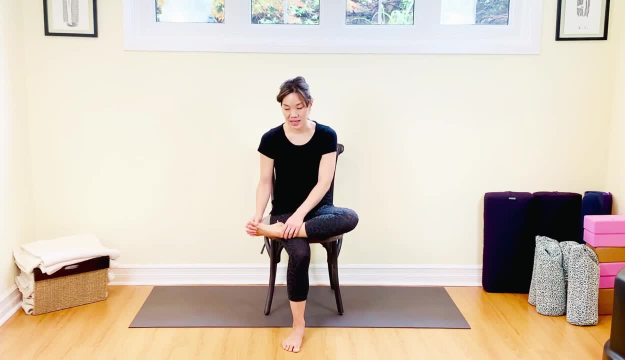 kind of a multitask here. We're rotating the joint of our ankle, We're also opening up our metatarsals, The toes, The spaces between those toes. Okay, So now I'm going to rotate the other way And of course, I'm breathing. A lot of times we hold our breath. 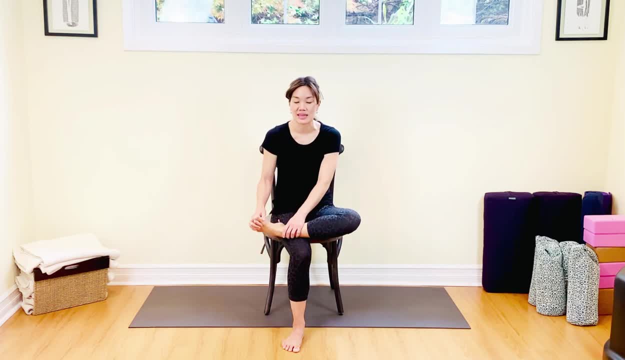 when we're concentrating on what we're doing. So try to breathe in and out. Okay, Now I'm going to release my toes. My fingers- Oosh, oosh, oosh, oosh, Shake out those fingers. Wiggle my toes. Now sit nice and tall. 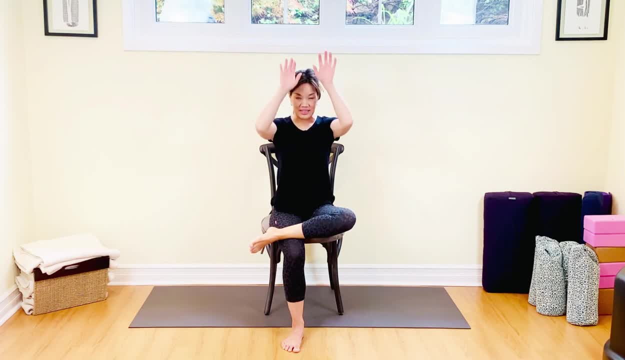 Breathe in, Breathe out. Hands down, Inhale. We're going to hinge at the waist, Lead forward with the chest And just when we feel like something is being stretched into this area and I'm feeling a little bit of a strain in my back, 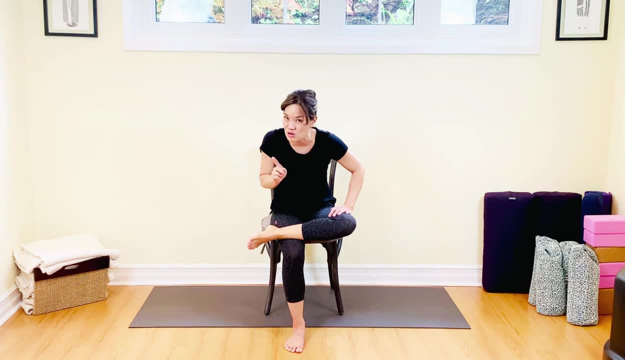 right away. I want you to round your back Right away. I want you to round your back, Round your upper back, so there's no strain on your lower back. Round the upper back and melt forward, Relaxing into the hips, Breathing. We're going to take two more breaths here, In and out: Inhale and exhale. 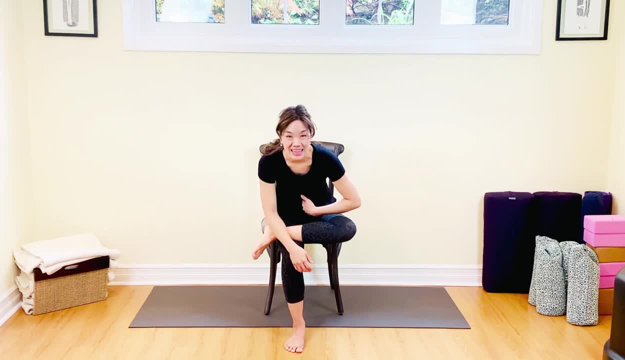 Very good, Slowly, Tight belly, Come on up Breathing in And exhale. See if you can cross your legs. so there's no window between those legs. Great, Let's go ahead for another twist. We're going to take that right hand, place it as you had done before. 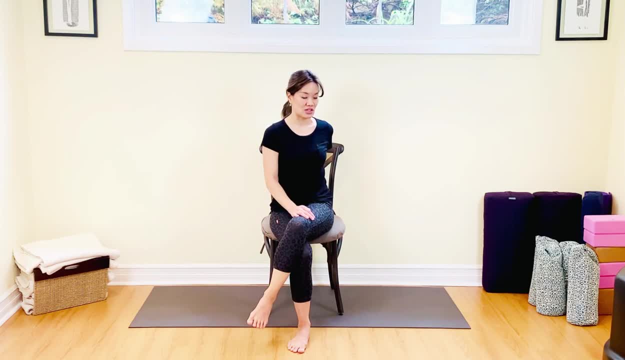 behind you on the seat, nice, and close to your sits. bones, Lift and lengthen, Breathe in here And then exhale, taking that left hand on the outer side of that right leg. Breathe in, Lift, Lengthen. 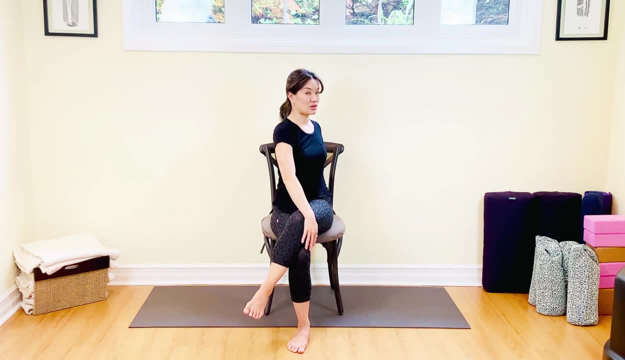 in lift, lengthen, then exhale, relax your hips gently, twist. so now we're going for a little bit deeper of a twist here, and only twist as much as you can or need to. okay, no strain. breathing in, exhale, breathe out, very good, inhale and then 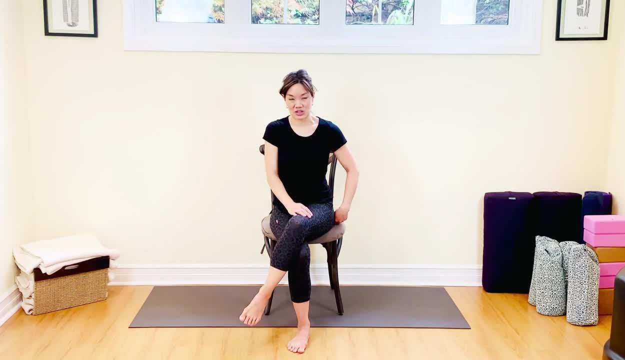 exhale, we're going to unwind, come back to center, back to neutral, and then slowly, with assistance, help that leg and switch. perfect, take your hands back to the chair, give these legs a little shake before we do the other side. okay, now take, taking that left knee up, nice sitting, nice and tall, and then exhale. 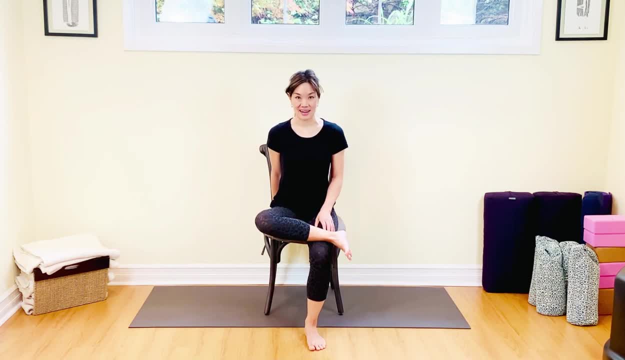 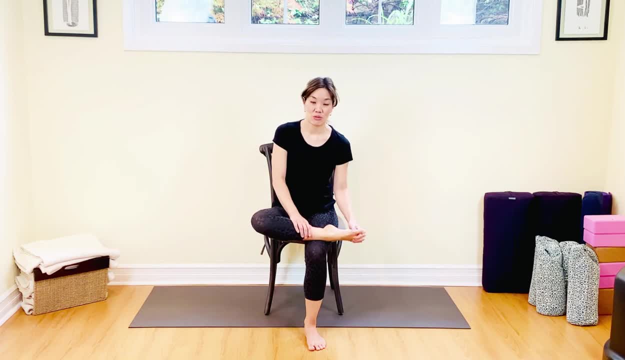 way and the other way with breath. okay, so go as slow as you need to, and I'm just gonna switch ways now. oh, my ankle just getting a little crack. there needed it needed, had to release some of that air between the joints, perfect, okay, now we're going to release those fingers, ah. 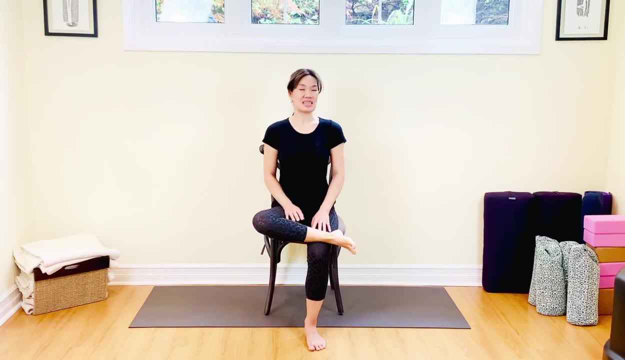 wiggle the fingers, wiggle the toes, sit nice and tall, breathe in, lift, lengthen up, exhale, release the hands down, now hinging at the waist again, we're breathing in and out. boom, a touch-up this hip on this side, such as to be a little bit more tight when I feel that. 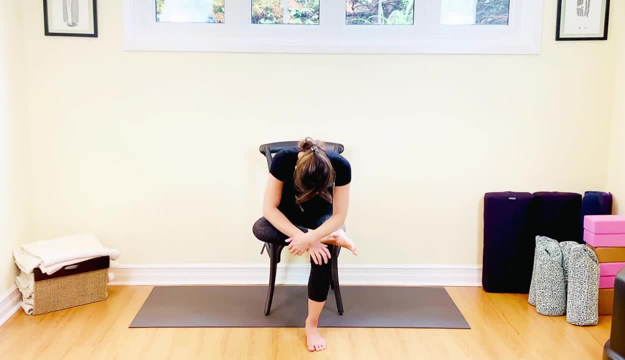 in this space. I'm getting a ride. cripple back and melt forward for two breaths. inhale here, exhale, inhale. well then, draw the belly in. so contract Oil's belly in a mantra. let your heart. último y no cinta, señor Wedding Hero. 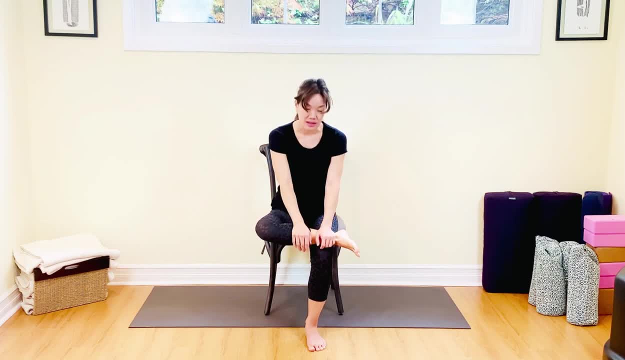 that one has to give me, and that's good Ravel, she into the hip flexor seaters contract those belly muscles to come on up, Inhale, lifting up and then exhale. Let's go ahead and lose that little window between the legs into a nice cross leg position, Perfect. Now let's go. 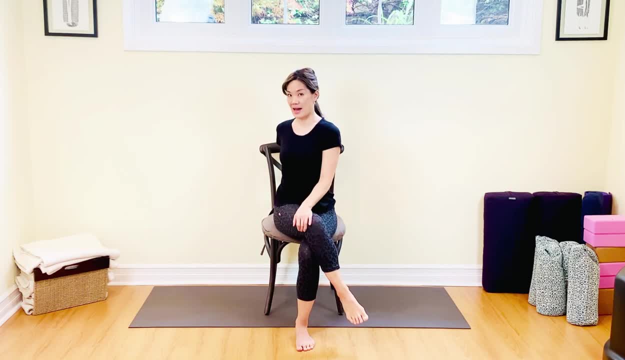 ahead and take our hand. So that's our left hand, behind nice and close to the sits bones, Breathing in. lift up with that right hand and exhale twist. Keep the chin right over the sternum, Breathe in. 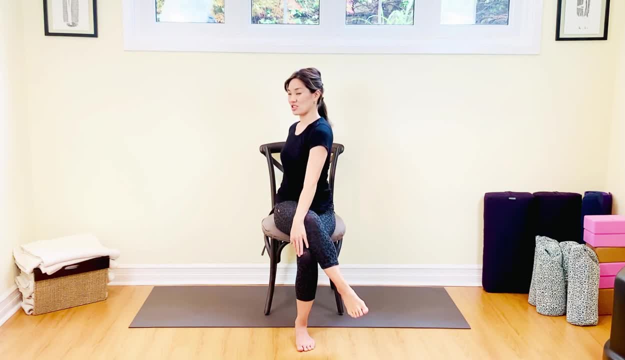 lift, lengthen and exhale twist. Relax your shoulders, relax those hips One more time breathing in and exhale twist: Very good. Inhale and then exhale, unwind, Breathe out.